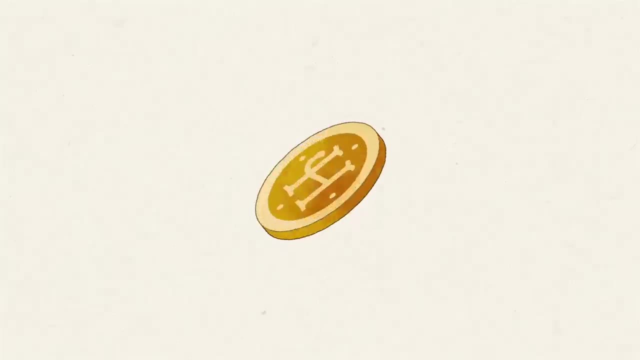 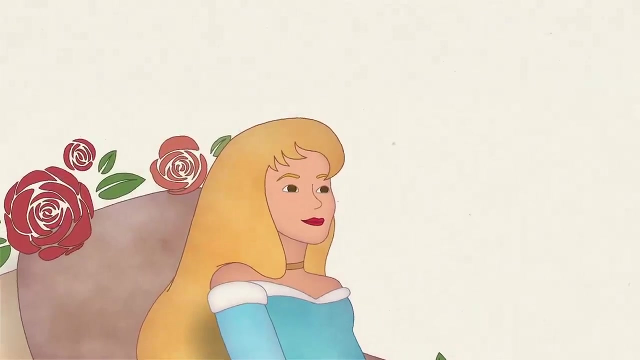 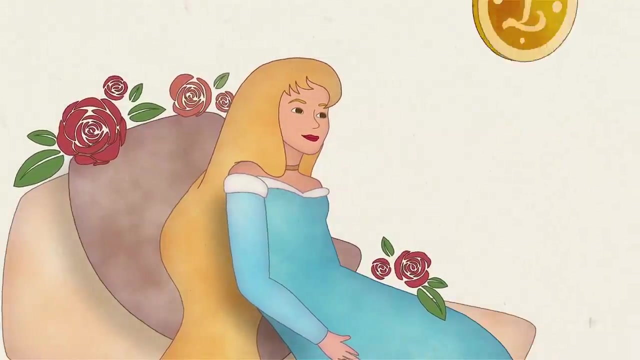 because she knows the coin is fair. Nothing changes between when the coin is flipped and when she wakes up, and she knew for a fact that she would be woken up and she receives no new information when that happens. Imagine that, instead of flipping the coin after she's asleep, the experimenters flip. 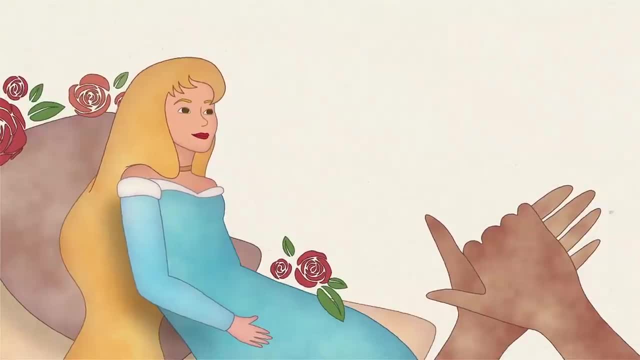 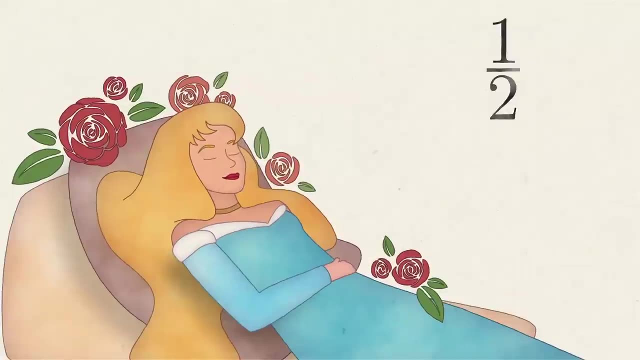 the coin first and ask her immediately what's the probability that the coin came up heads? Well, she would certainly say one half, So why should anything change? after she goes to sleep and wakes up? This is known as the halfer position. 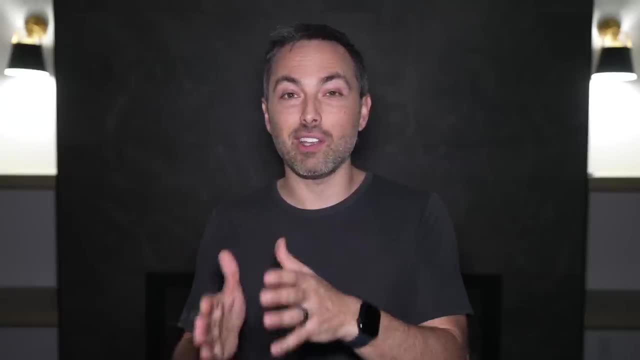 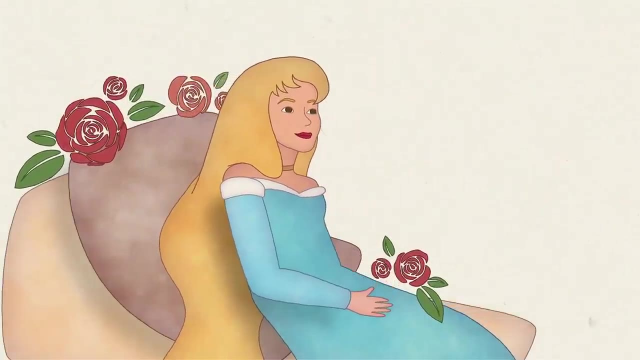 But there is another way to look at it. Others would argue that something does change when she's awakened. I mean, it seems like she gets no new information. there are no calendars, no one tells her anything and she knew that she would be woken up. but she actually learns something important. 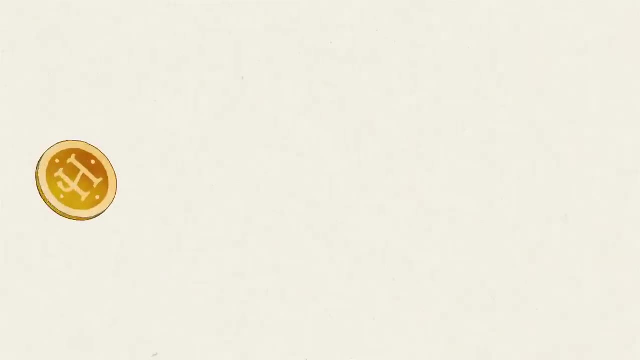 She learns that she's gone from existing in a reality where there are two possible states. the coin came up- either heads or tails, So she's awake. There are three possible states in the Patientenjes: either heads or tails, as previously mentioned. 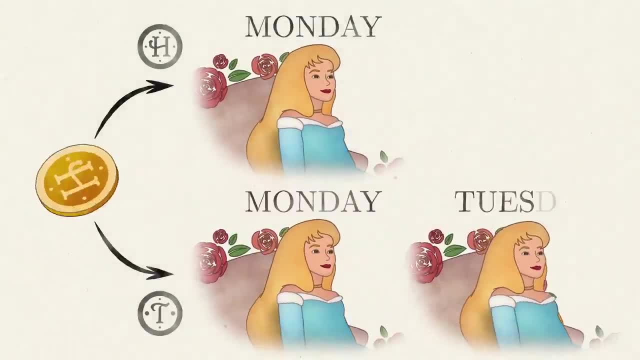 You can see, all theseinski cells are connected in stronger arranged order and altering the Watchmen general situation. The reality of the Bitcoin coin, though, naturally has beenاث Monday heads, Monday tails or Tuesday tails. Therefore, she should assign equal probability of soithes three outcomes, even if the heads 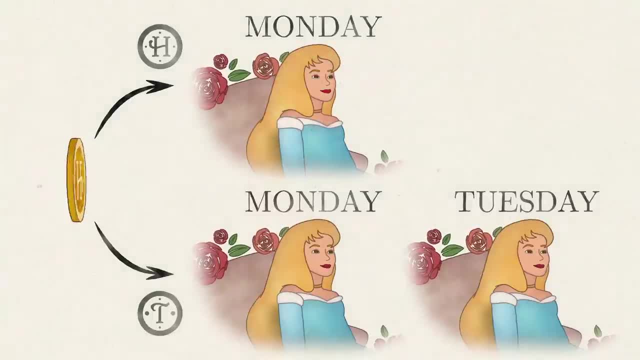 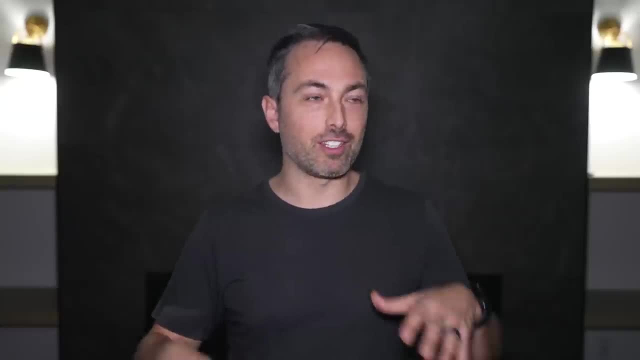 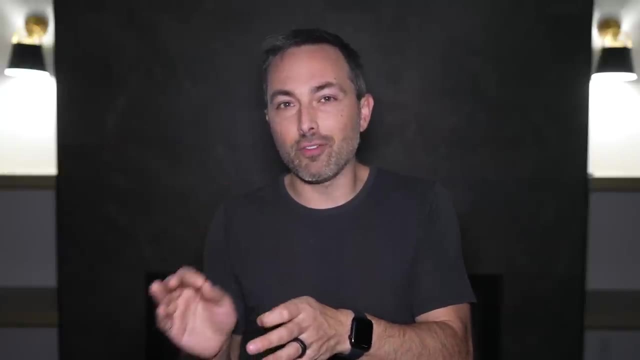 were in one. So the suggest that a fair coin should have a one third probability of coming up heads- but that's because a dónde You're still thinking about this- is subtly different. The implied question is: given you're awake, what's the probability that? 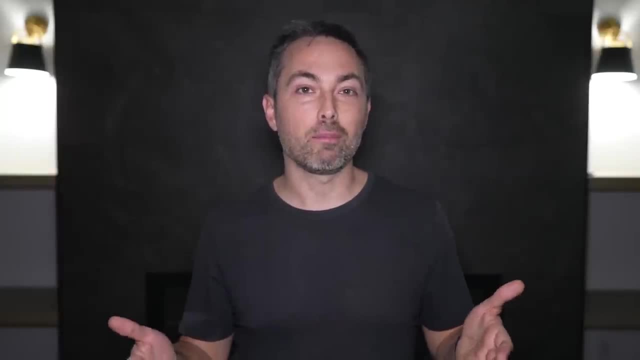 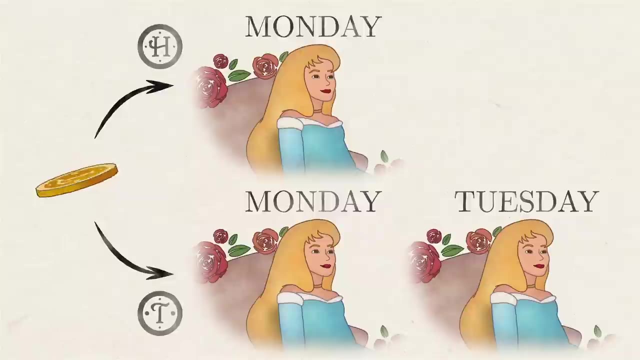 the coin came up heads, And that is one third. Now halfers would counter that just because there are three possible outcomes doesn't mean they are each equally likely. In the Monty Hall problem, for example, the contestant ultimately has to choose between two doors. but it'd be wrong. 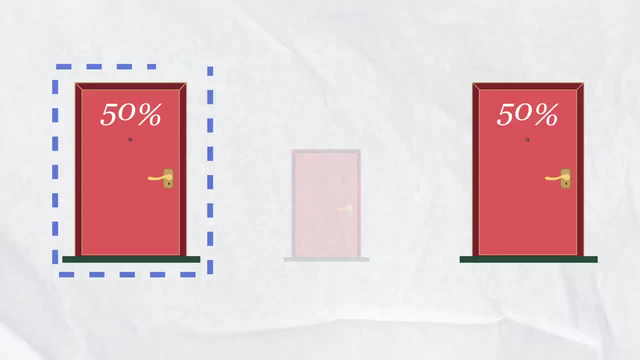 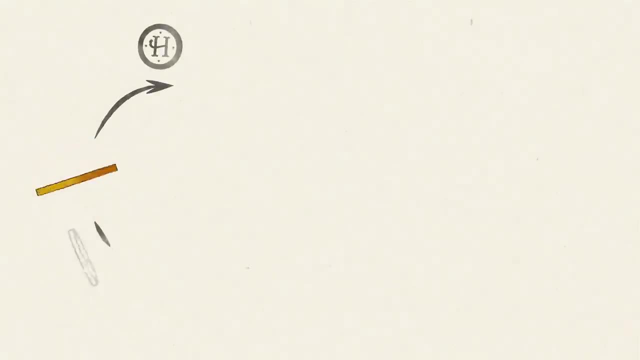 to assign them 50-50 odds. The prize is actually twice as likely to be behind one door than the other. In the Sleeping Beauty problem we know a heads outcome and a tails outcome are equally likely. so the chance of waking up on Monday with heads is 50%, and the chance of waking up on 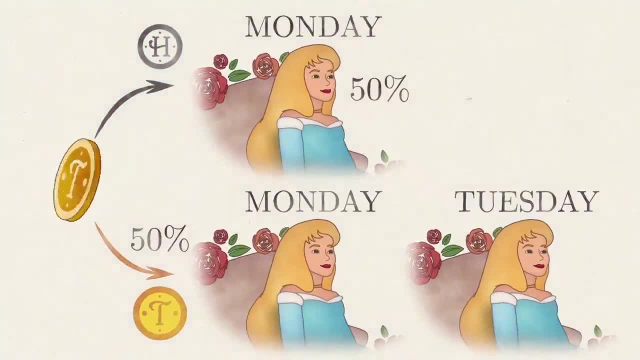 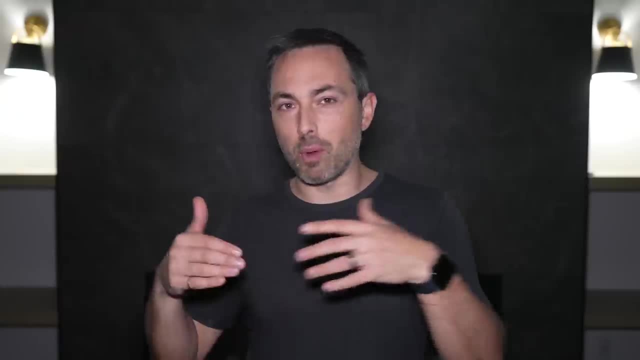 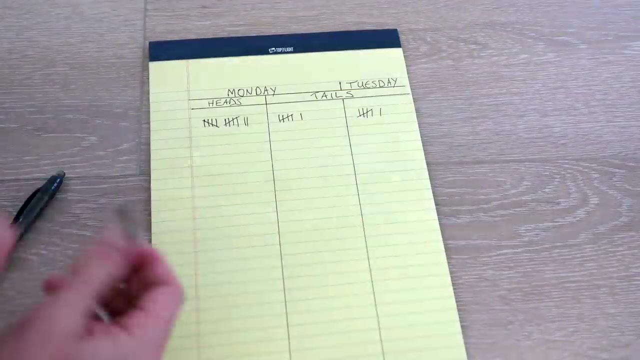 Monday or Tuesday with tails should be 50%. Therefore the tails probability gets split across two days, 25% each. But if you repeat the experiment over and over, which you can try for yourself by repeatedly flipping a coin, you find she wakes up a third of the time. Monday heads. 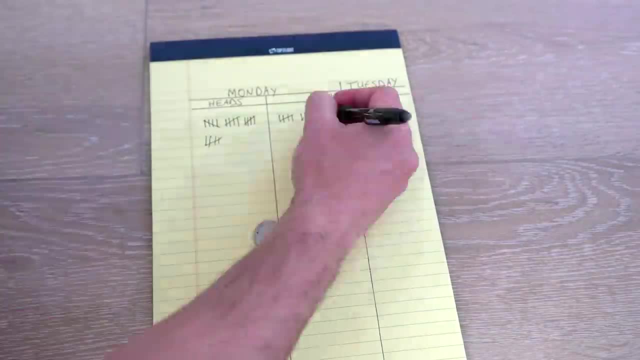 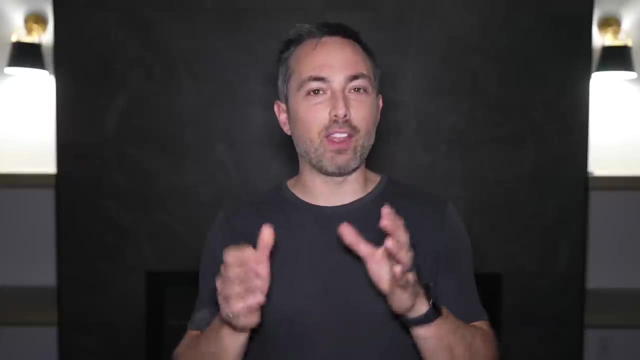 a third of the time Monday tails and a third of the time Tuesday tails, not 50-25-25, like the previous analysis would suggest. So if you were Sleeping Beauty and you were awakened and asked what's the probability, the 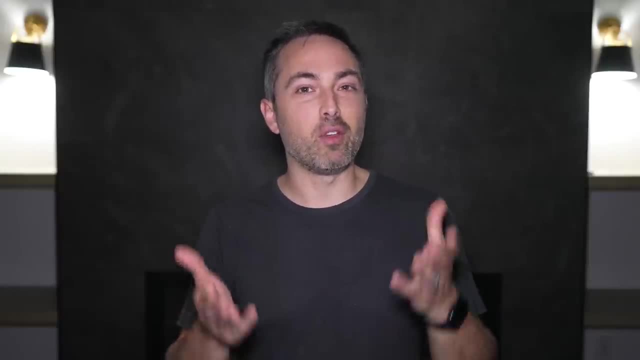 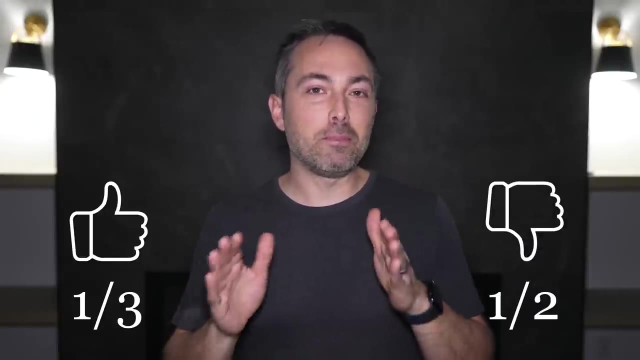 coin came up heads. what would you say? If you would say one third, then hit the like button. If you would say one half, hit the dislike button. The answer may seem obvious to you, but you should know that to other people the other answer seems equally. 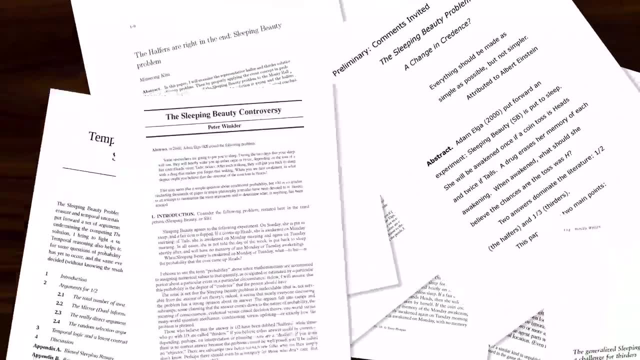 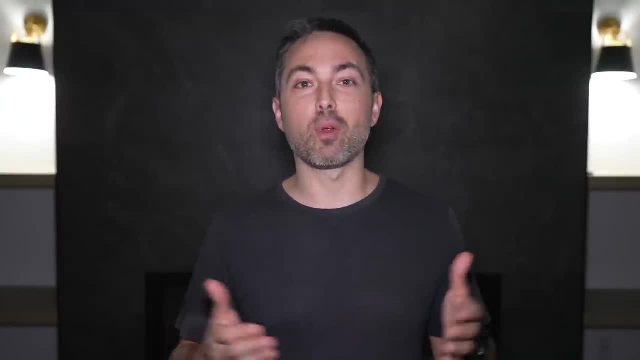 obvious, the fact that you are not sleeping. beauty is probably not the right answer in the obvious, and that's why hundreds and hundreds of philosophy papers have been published on this problem over the past 22 years. There have been many variations of this problem, like: what if, instead of being woken up twice, 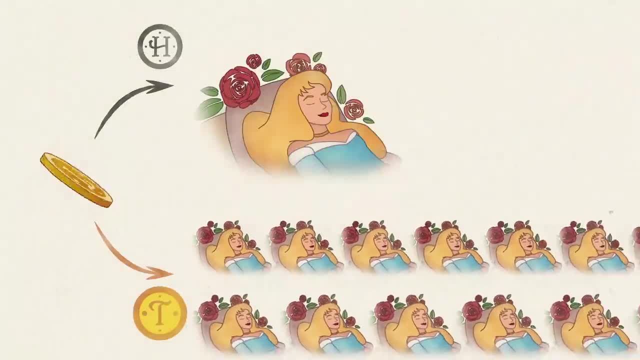 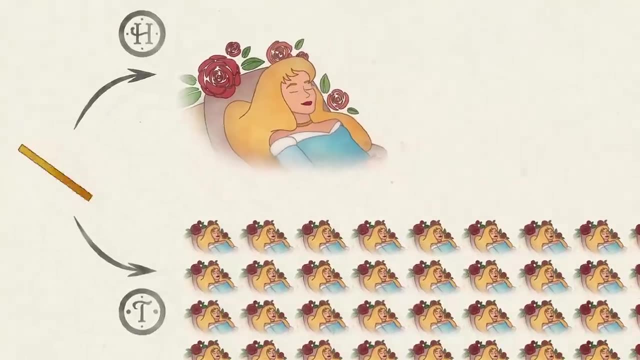 if the coin lands tails, she's instead woken up a million times. If the coin comes up heads, she's still woken only once. Doesn't it seem absurd in this case when Sleeping Beauty wakes up to say that it was just as? 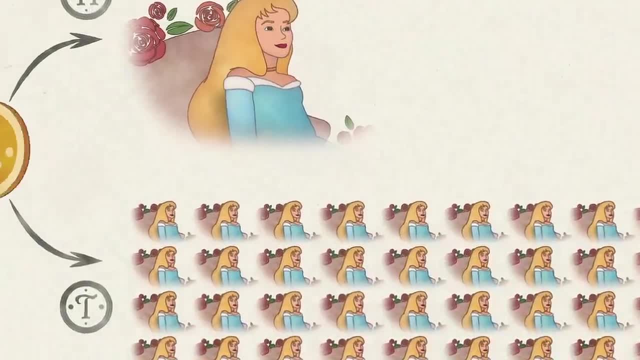 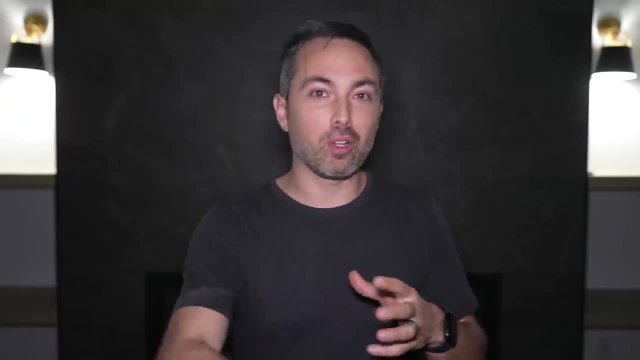 likely that the coin landed heads as tails And we know there are a million more wake-ups in the tails case than in the heads case. If you reach into a bag of one white marble and a million black marbles, what are the chances that you pull out that one white marble? 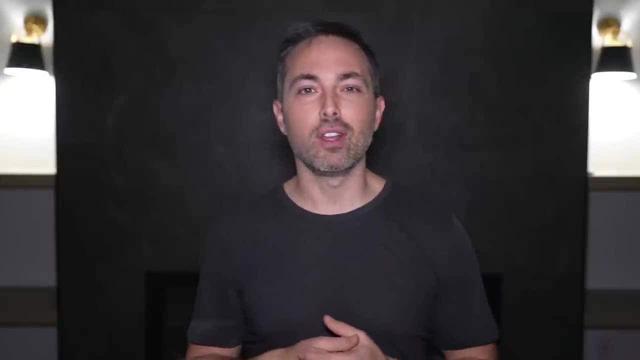 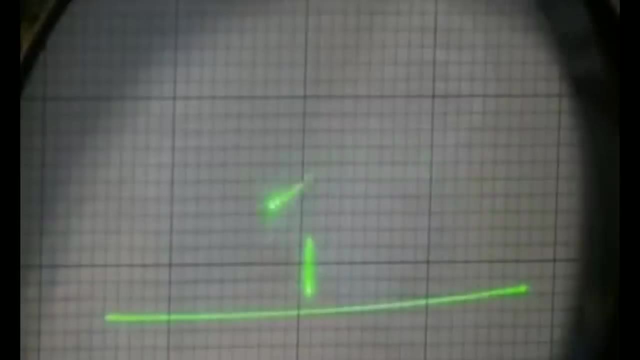 I was pretty convinced by this and I considered myself a thirder. but this same argument is used to convince people that we're living in a simulation. The thinking goes that our computing technology has improved so dramatically, even over just the last 40 years, that we can imagine a time in the not-too-distant future when we can. 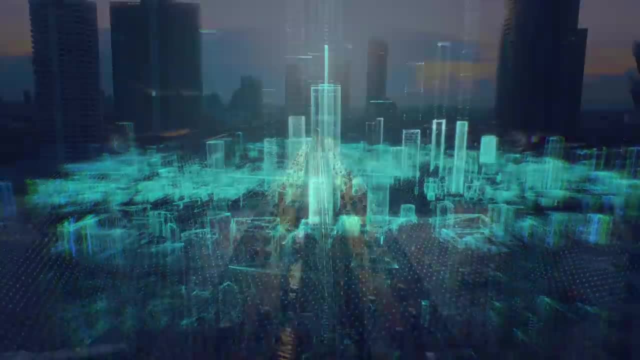 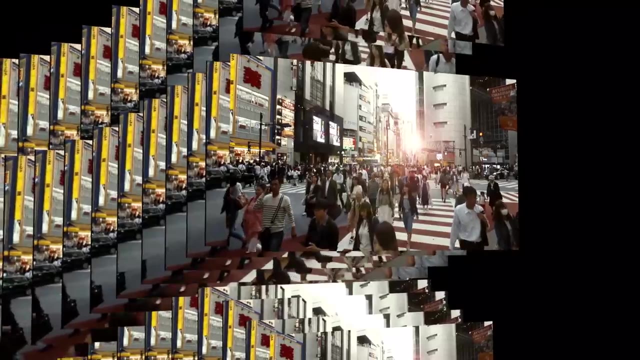 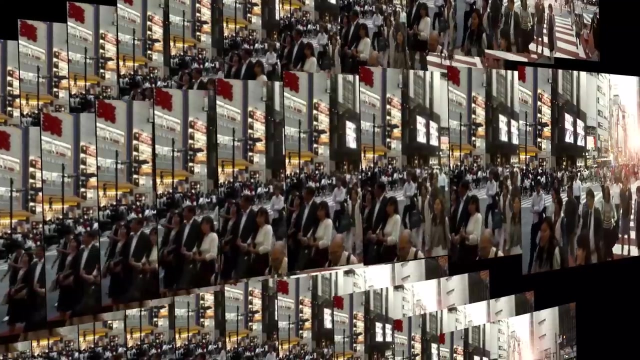 create a completely realistic simulation of our world, And once that occurs, it should be trivial to make unlimited copies of that simulation. And then if you were to ask someone if they're living in a simulation, they would have to admit that they probably are, because there are many more instances of that existence. 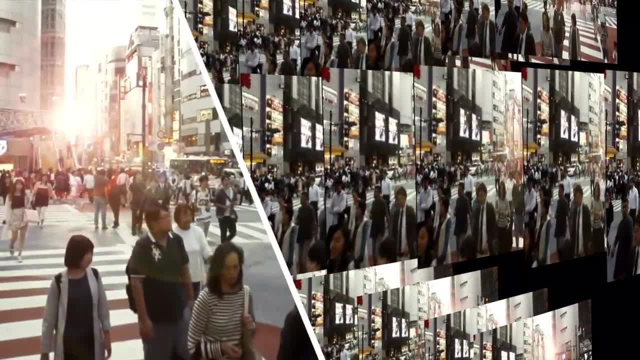 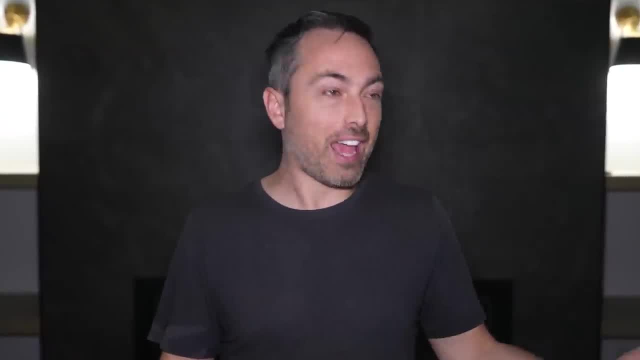 than the one true external reality. But how do we know that this hasn't happened already and that we're living inside a simulation? I mean, if it can happen, then it probably has happened And we are living in a simulation. This seems like the logical conclusion of the thirder worldview. 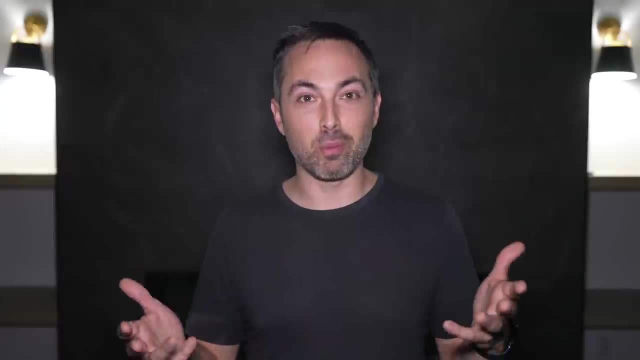 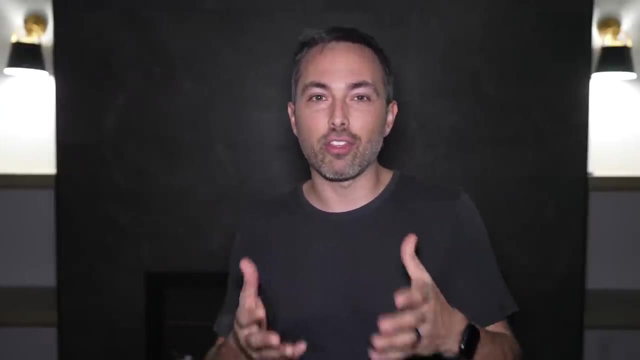 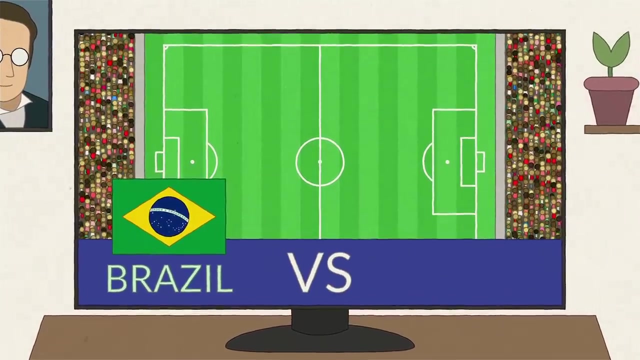 Now I personally don't buy that. I'm living in a simulation and I think most people don't buy it. but maybe that's just illogical bias. But there's another thought experiment that makes me seriously reconsider the thirder position. Let's say there's a soccer game between a really great team like Brazil and a less world-dominating 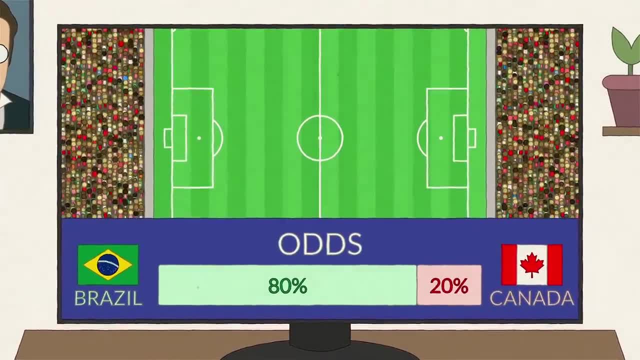 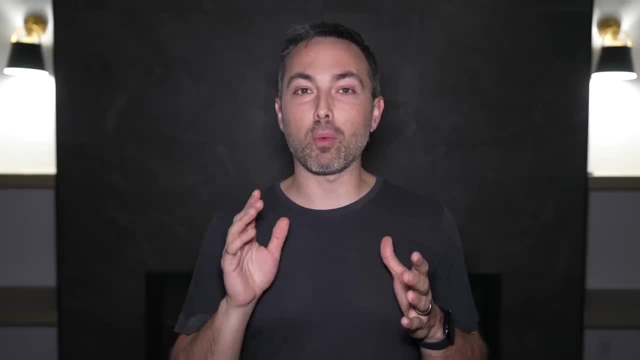 team like Canada. So the odds are 80-20 in Brazil's favor And it's going to put you to sleep before the game starts, And if Brazil wins they'll wake you up one time, But if Canada wins they'll wake you up 30 times in a row. 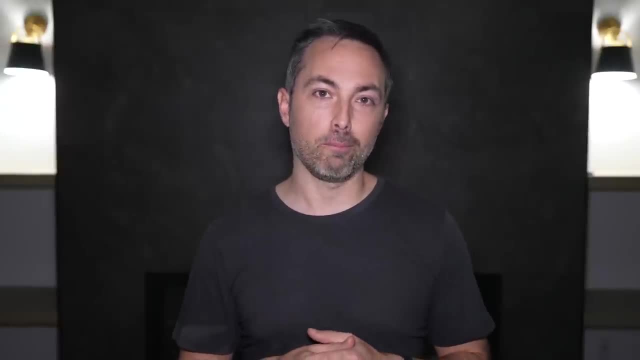 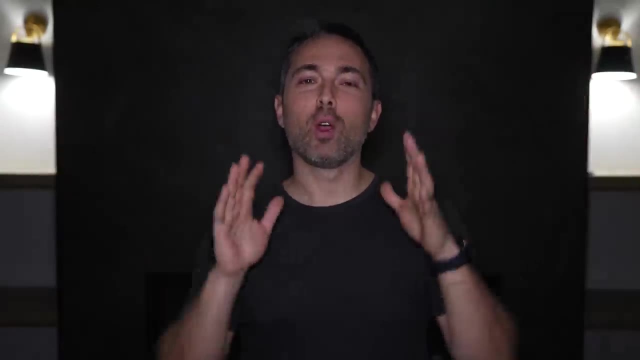 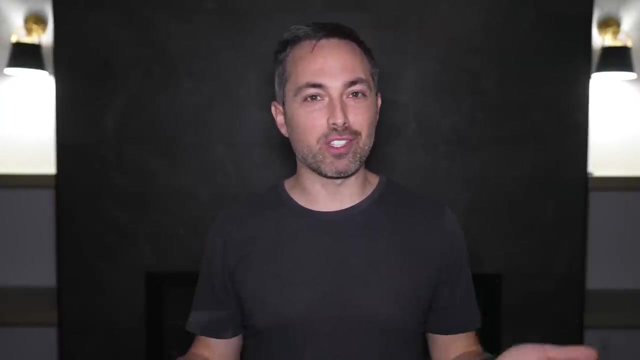 And, just like Sleeping Beauty, you won't remember if you've been woken before. Okay, so the game is about to start. you fall asleep and now you're woken up. Who do you think won the game? The thirder would say Canada, but I would almost certainly say Brazil. 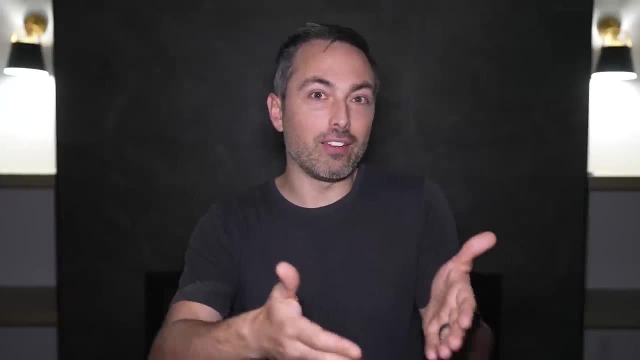 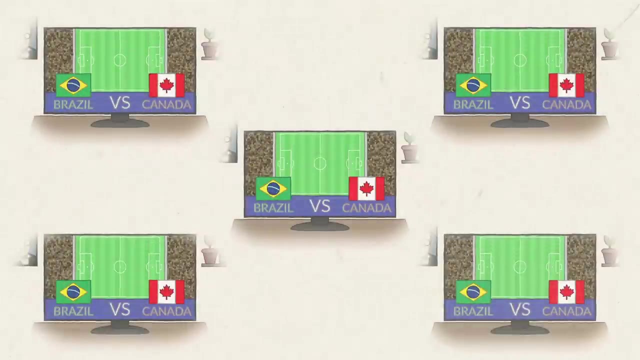 I mean, why should I give any weight to what the reason is? I mean, what would a researcher have done if Canada had won, when I'm fairly confident that they won't? To extend this, let's say Brazil plays Canada five times and we do this experiment each. 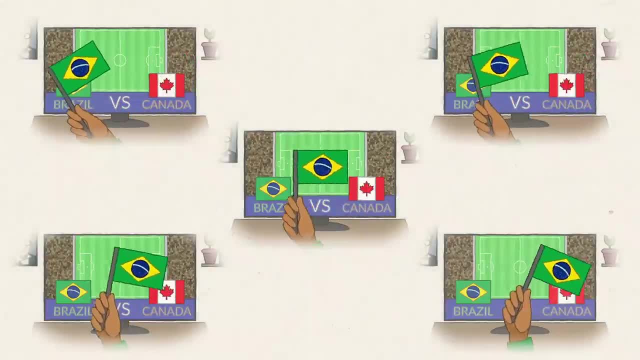 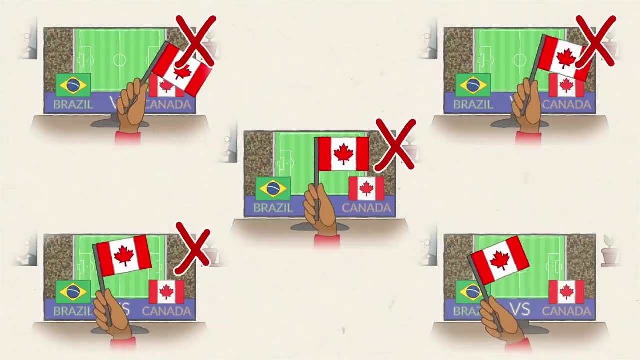 time. Well then, if you say Brazil each time, you're woken up, you'll probably be right about four out of five of the games, But if you said Canada every time, you would be wrong about those four games, but right 30 times in a row when you're repeatedly asked about Canada's one victory. 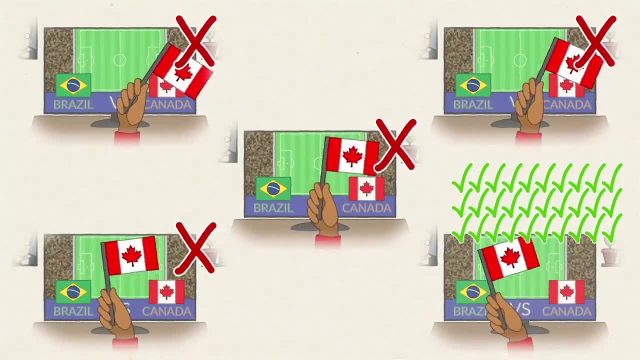 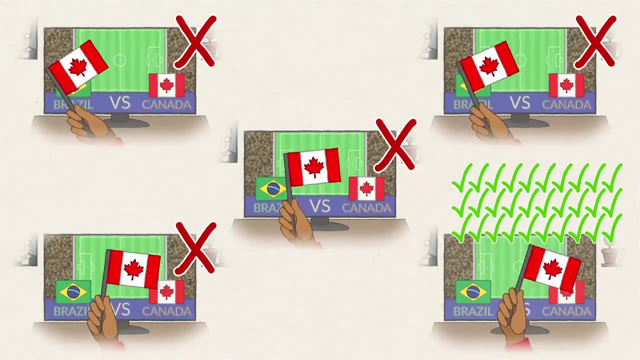 If you stand to win a bet by correctly answering the question, Then by all means you should bet on Canada, But if you want to correctly pick the winner of more of the games, well then you should say Brazil. And this is what's at the heart of the dispute between halfers and thirders in the Sleeping. 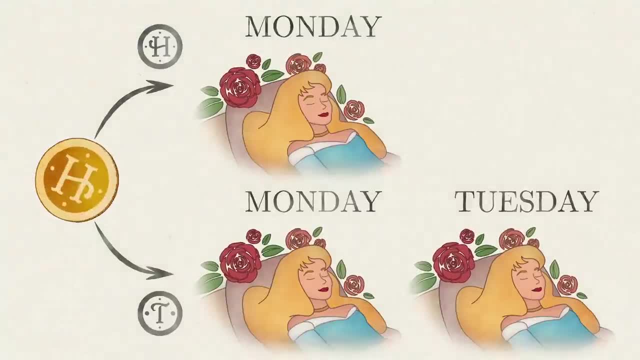 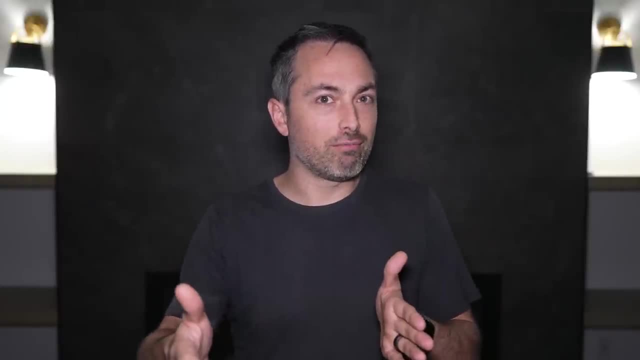 Beauty problem. If you want to be right about the outcome of the coin tosses, well, you should say the probability of heads is a half. But if you want to answer more questionings correctly, well then you should say one third.